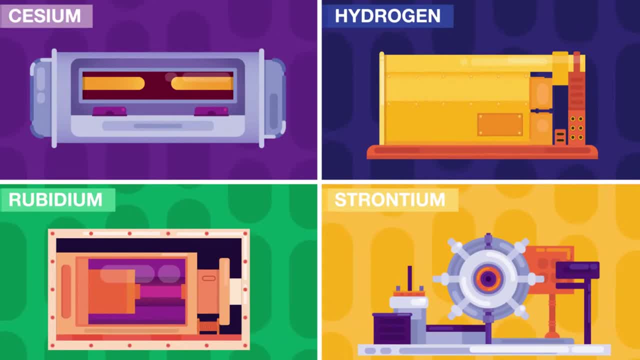 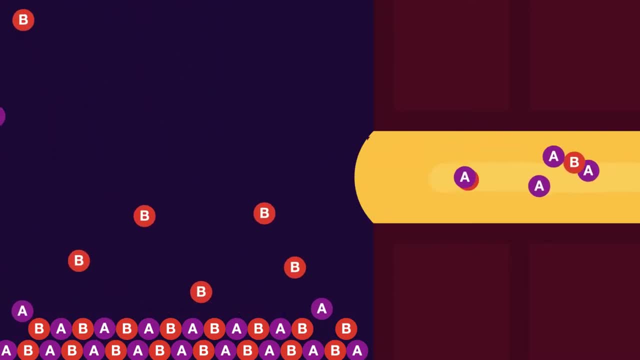 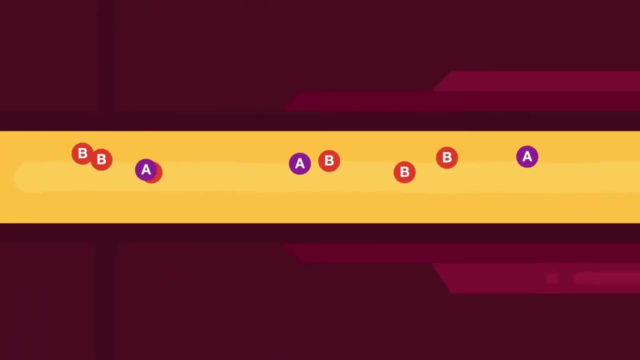 which is the same principle as the oscillation of an atom. All the different types of atomic clocks commonly share the same working principle. Initially, the atoms are heated in an oven prior to their bundling into a beam. There are two possible energy states or hyperfine levels in each atom, namely state A and B. In this step, 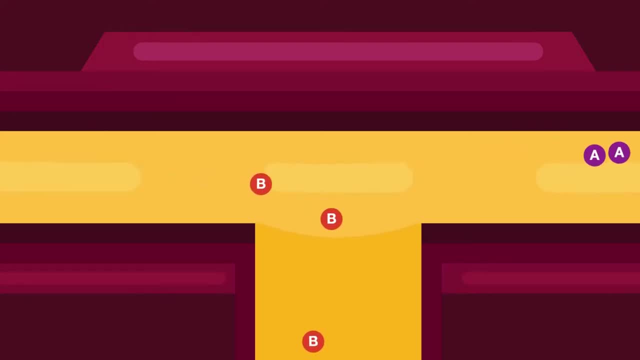 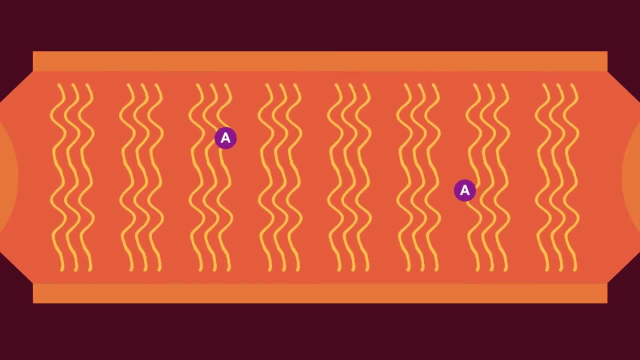 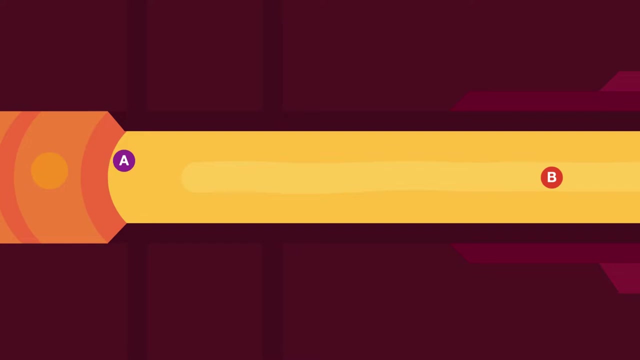 atoms in state B are eliminated by a magnetic field, while atoms in state A remain in the beam. In the second step, the state A atoms are exposed to microwave radiation by sending them through a resonator. Due to this radiation, some of the state A atoms are shifting to state B. A second magnetic field is then fired. 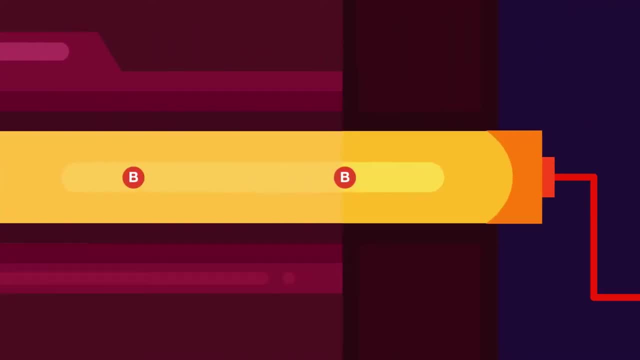 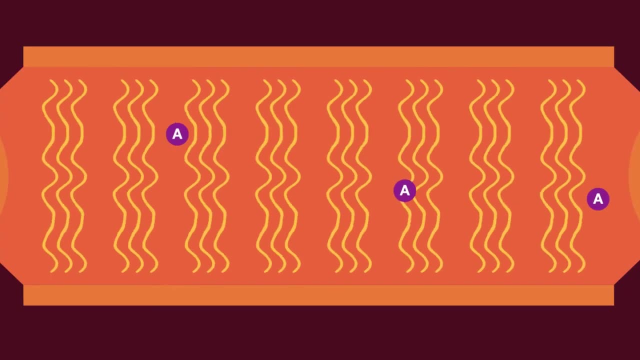 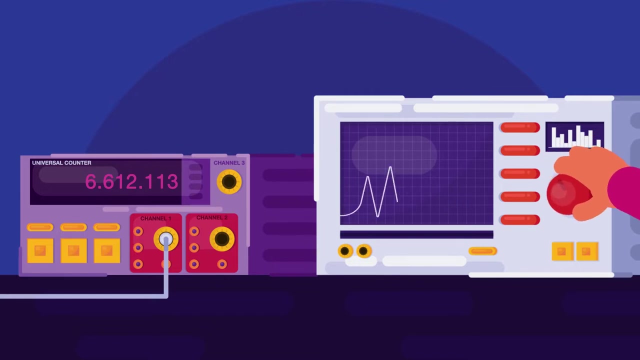 to eliminate atoms that are still in state A. The remaining shifted state B atoms are then counted using a detector. The frequency of the microwave radiation determines how many of state A atoms that can be shifted to state B atoms. The more synchronization events happen between the frequency of microwave radiation and the state B atoms, the more 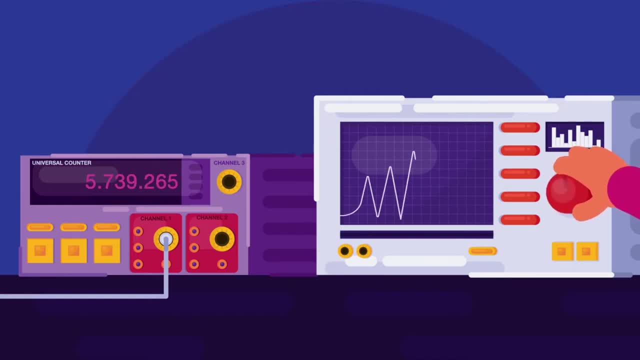 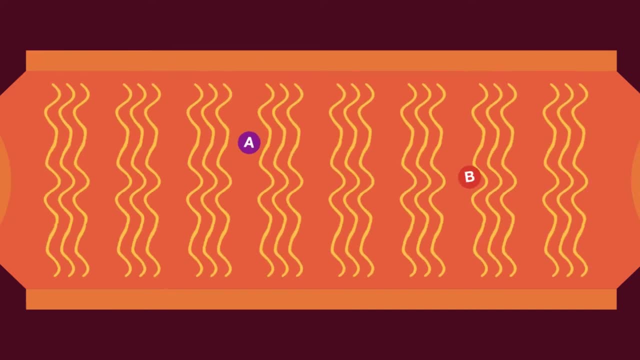 atoms can be shifted into state B atoms. In fact, the purpose of this step is to adjust the microwave radiation frequency to match the frequency of oscillation of the atoms In the nine billion, one hundred and ninety-two million, six hundred and thirty-one thousand. 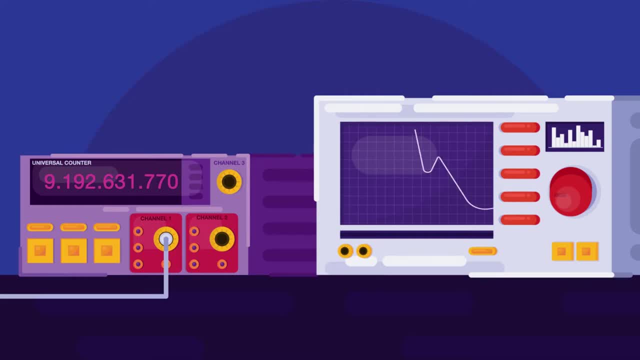 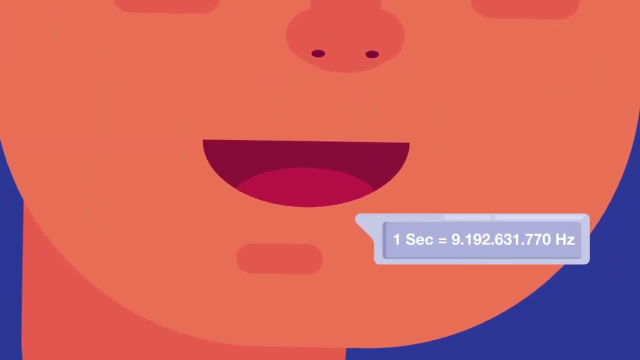 seven hundred and seventieth oscillation of the atoms. it is defined as one second. The Meowth Number of Oscillations, The lol Number of oscillations, gives us an idea of how accurate the atomic clock is. The atomic clocks are so accurate that they. 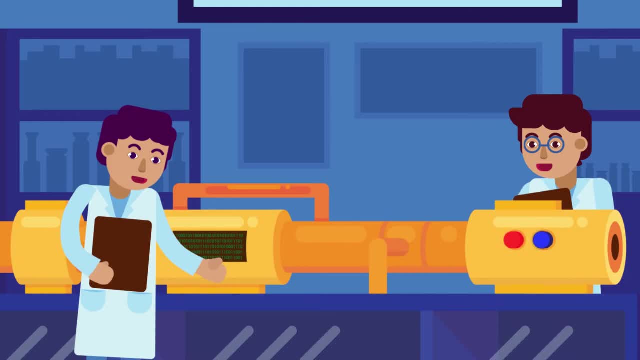 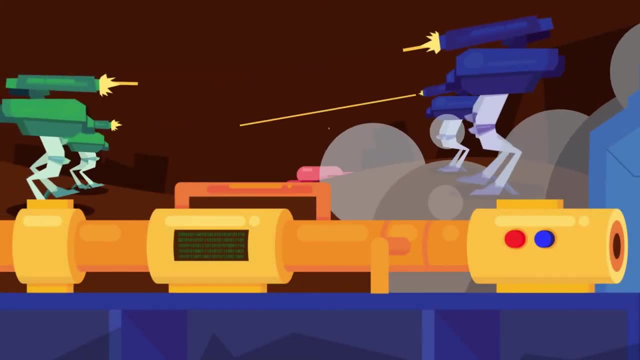 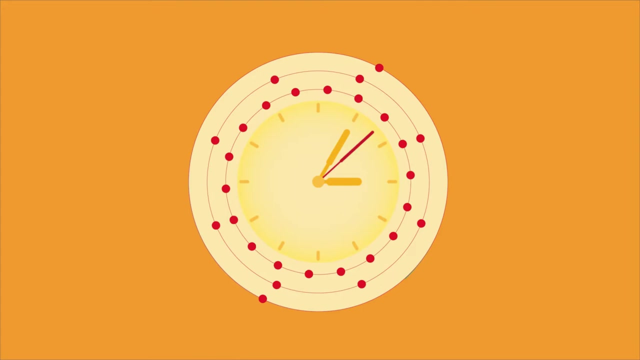 are known to make a one-second error in about …. Can you guess If you guessed one hundred or two hundred thousand years? that is incorrect. The clock is known to make a one-second error in about ten million years. So how many of this atomic clock exist worldwide? 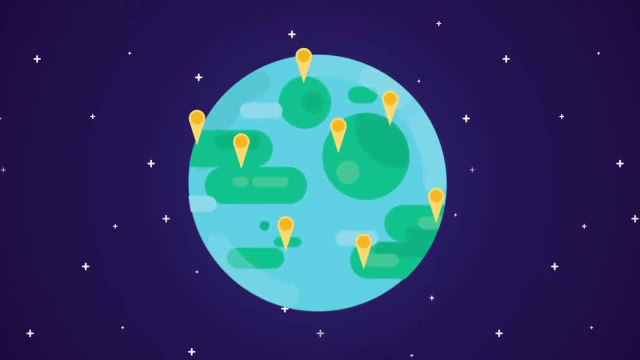 Quite a lot, actually. So far there are four hundred of these clocks worldwide. Has the atomic clock add home every哪些天份 pre Clint Eastwood ran得 他們其中十万年 year in the nuclear field, So they must be an unchanged number of that time. 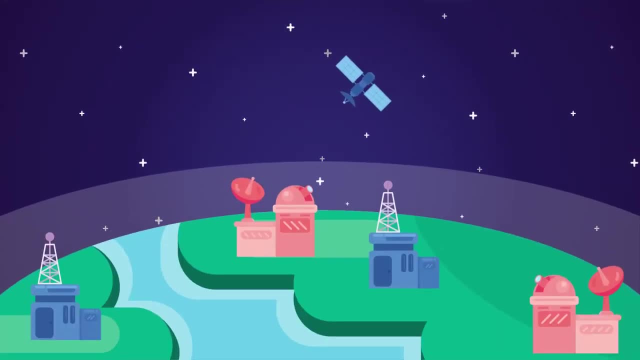 Since the atomic clock may be the first galaxy that has ever 가. binge�도 определ heed to an ultimately worldwide, owned by around 70 meteorological institutions and observatories, and are used to determine Coordinated Universal Time, or more famously known as the UTC and local.